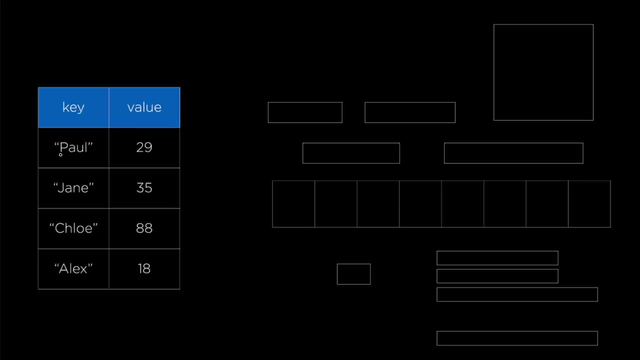 the first character of each key and compare it to the letter A And compute how many characters away it is from the letter A. So, for example, for this key, Paul, you can look at the first letter P, convert it to the lowercase p and compare it to the lowercase a. 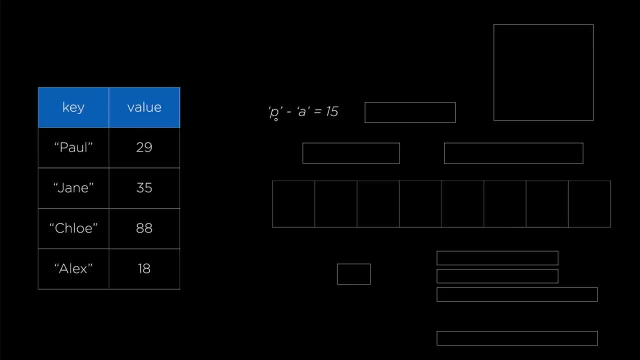 And in ASCII code you'll be able to see that P is 15 characters away from A. But 15 wouldn't be an index of this array because that would be out of range. So you would need to use, for example, the mod operator, mod8, mod of the length of the array. 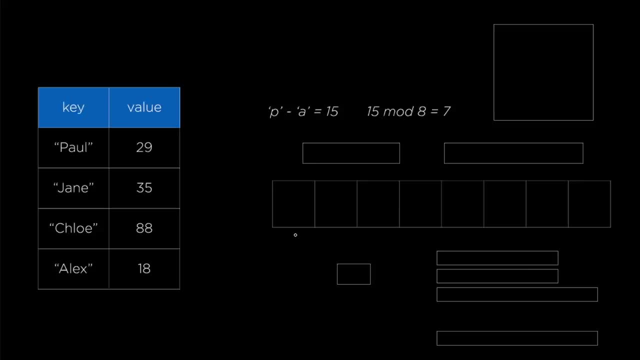 to get the desired range, That would be 0 to 7 inclusive. With that method you would get 7.. So at that point you can put this key-value pair- Paul29, over here at index 7.. And just like that we can decide which index of the array we want to use. 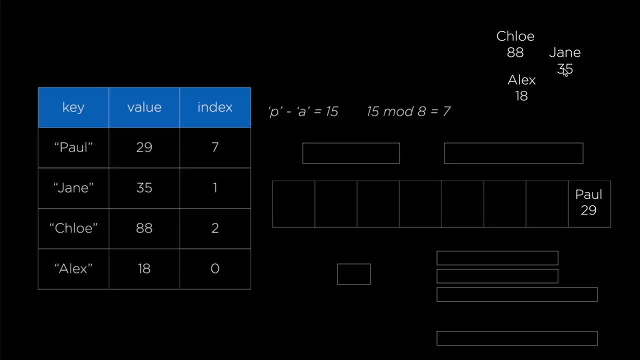 for each key-value pair. So Jane would be over here at index 1.. Chloe would be over here And Alex would be over here, And actually what I showed you here is already a hash table. So, basically, to construct a hash table, 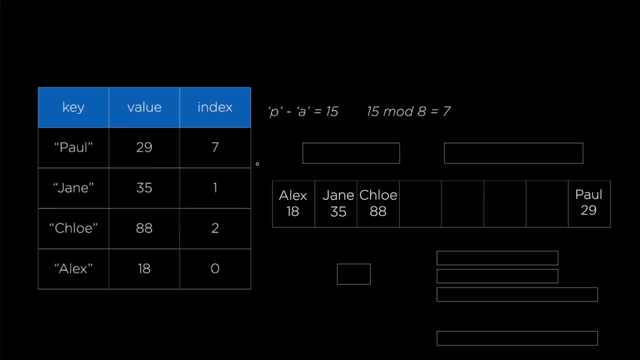 you need an array and a dictionary you want to represent and a way to decide which index of the array you want to use for each key-value pair. Another way to describe the same thing would be to say: we need a function that turns each of these keys. 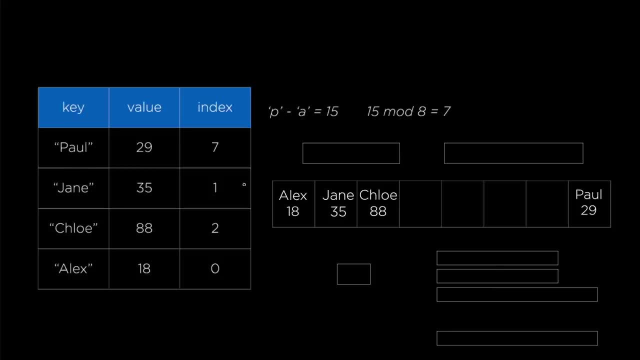 whether they're strings or anything else- into an index of this array that we constructed And we could call that function, for example, h1,. with the method that I just showed you, h1 of Paul would be 7. And this function is usually called a hash function. 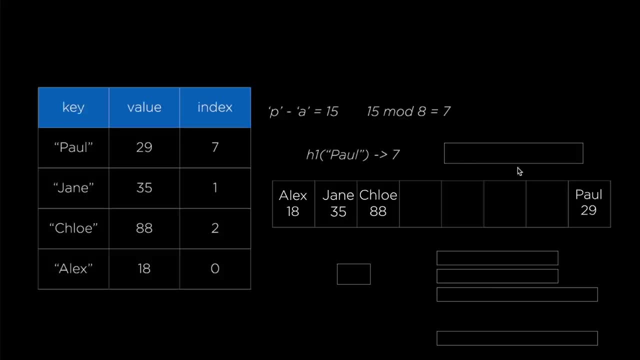 and that's why this whole thing is called a hash table. But this particular hash function that I just showed you might not be ideal for a few reasons. One of them is this: If you consider English names, there might be a lot of names that start with J. 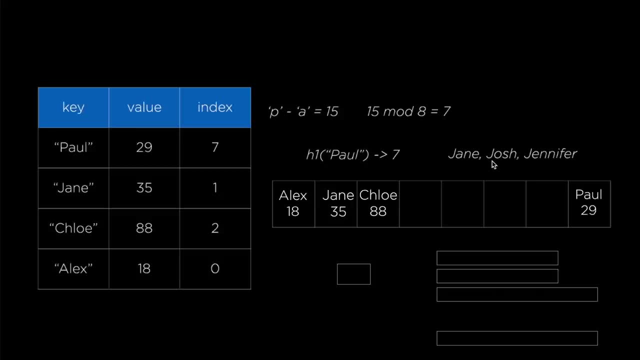 And if you put, for example, Josh in this dictionary or this hash table, it would try to go into the same bucket as Jane and the same thing with Jennifer, And that would be called a collision, when multiple keys would try to go into the same spot. 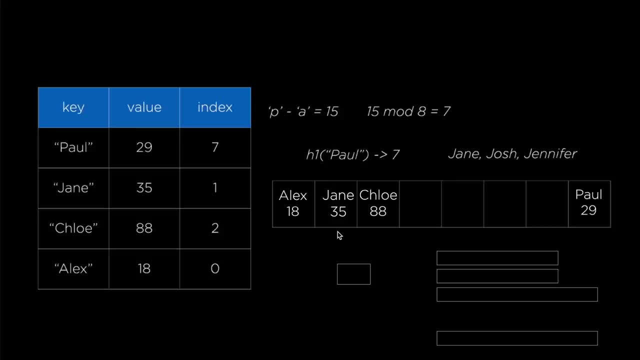 of this array, And there is a way to deal with collisions, and we're going to talk about those, But for now, you should know that we want to avoid collisions as much as possible to keep your hash table efficient, And so one way to deal with a problem like that. 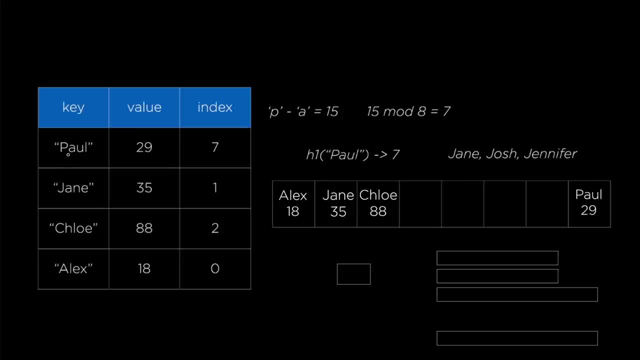 would be to consider most of the letters, or many of the letters, in the given key, if not all of the letters, And one such function is called djb2.. And I'm going to put a link to some information about that in the description, just in case you're curious about it. 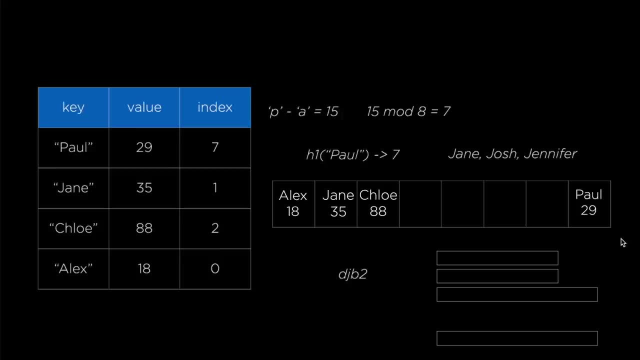 Anyway, when you're choosing a hash function for your hash table, there are a few things that you should consider. One is that it should be fast to compute, And the other one is that it should try to avoid collisions as much as possible. 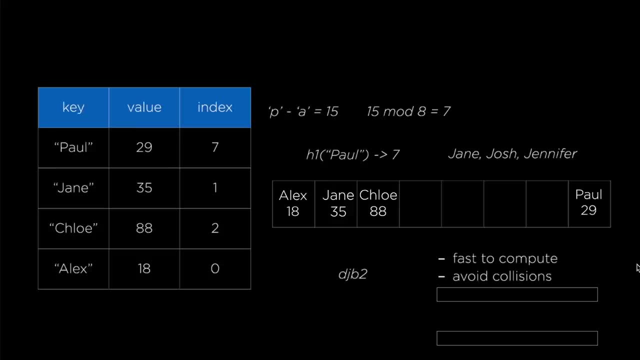 And that's pretty much it when it comes to the criteria. In some textbooks they might say: your hash function should be uniformly distributed or randomly distributed, Random looking or something like that. But it's really not necessary for practical purposes And it's not necessarily better than. 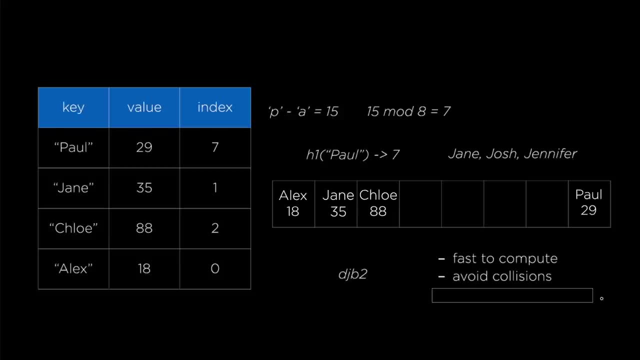 non-uniformly distributed functions. So if you're choosing a hash function for your hash table, you should really only consider these two criteria, And when you're choosing a hash function for security purposes, you might have other concerns, But here we're only talking about. 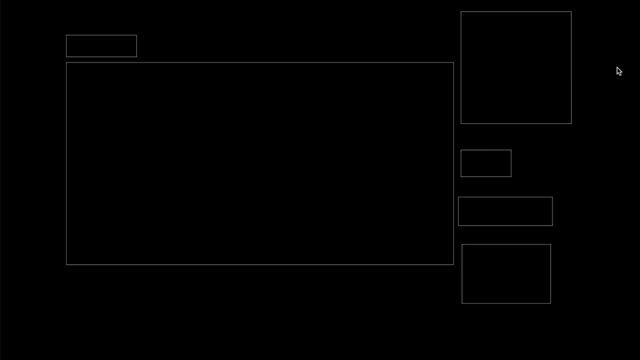 a hash function for a hash table. Okay, let's now talk about how to deal with collisions. We're going to talk about two families of methods for dealing with collisions in this video, And the first one is called chaining With this method instead of storing. 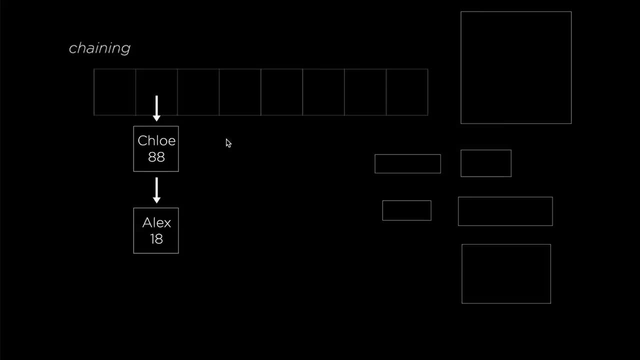 the key value pairs directly in the array. we're going to store them in a linked list And from each element of the array we're going to have a pointer to that linked list And that linked list is going to contain all the key value pairs that were assigned. 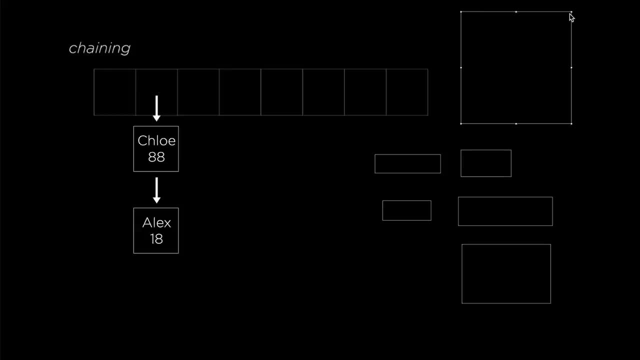 to that particular slot in the array. So, for example, if you have another key value pair that was assigned to this same slot, then what we'll need to do is we'll need to put the new key value pair at the beginning or at the top. 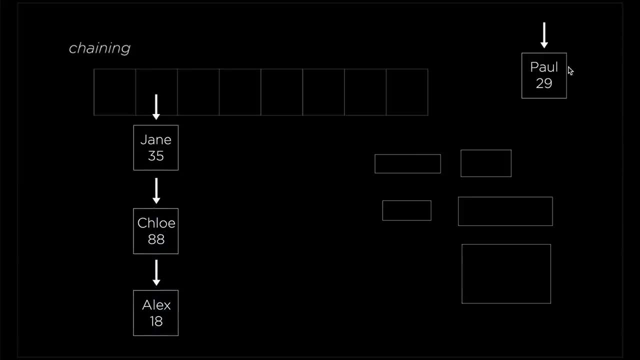 of this linked list, just like that. And if you have another key value pair that was assigned to an empty slot, then we'll need to create a new linked list containing this single element and then have a pointer that points to the new linked list from that slot. 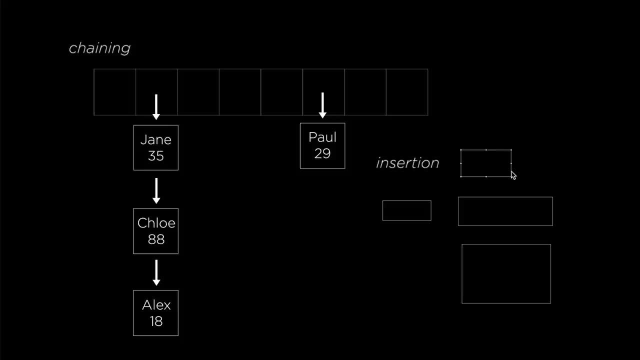 And with chaining, insertion only takes O in time or a constant amount of time. And what about search? Well, to explain that, I'll need to first define a few variables. n: here is the number of elements that we have put in so far in this hash table. 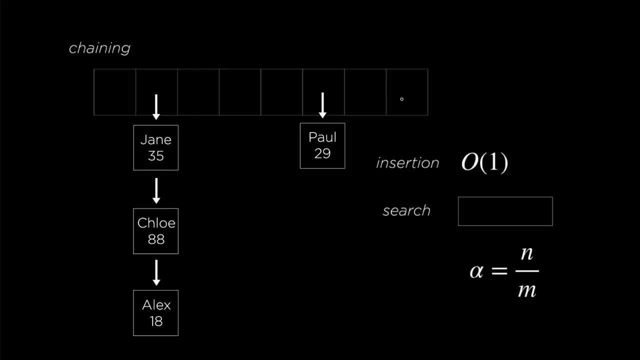 And m is the length of the array. So this alpha, which is n over m, is going to show how full this hash table is. So right now, because n is 4 and m is 8, alpha is exactly a half. 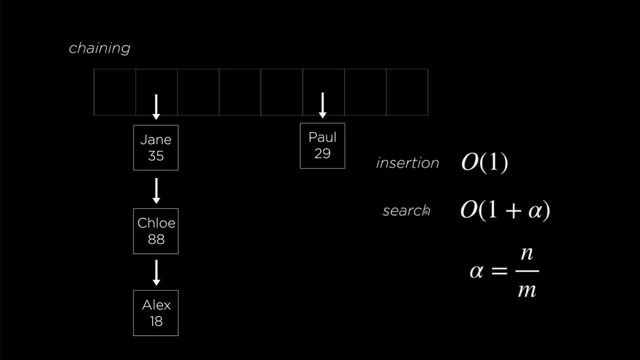 And with this you can show that search only takes O in time. What this means is that if you keep alpha below a certain number- below, let's say, 1, search would only take a constant amount of time, And this O is the average time. 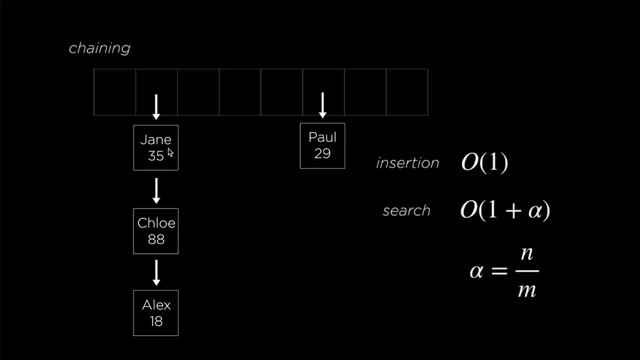 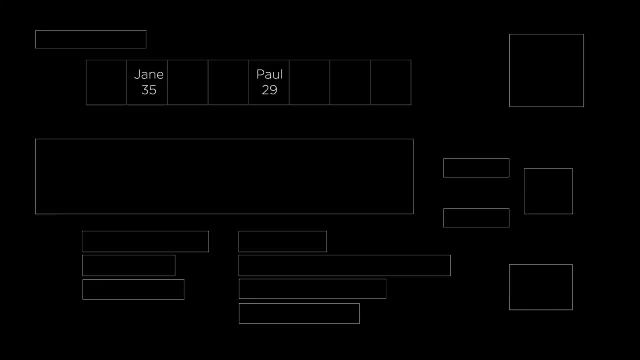 And here you might say: what if I don't want to use this extra data structure outside of this array? Then the approach you might want to use is called open addressing, And there are a few different flavors for it. I'm going to explain the simplest one first. 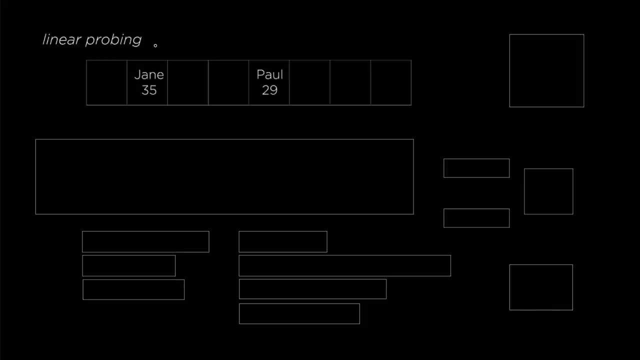 which is linear probing, With linear probing or with open addressing? in general, we store all the key value pairs within the array itself, just like you can see here. Let's say here that we have another key value pair that collides with this one. 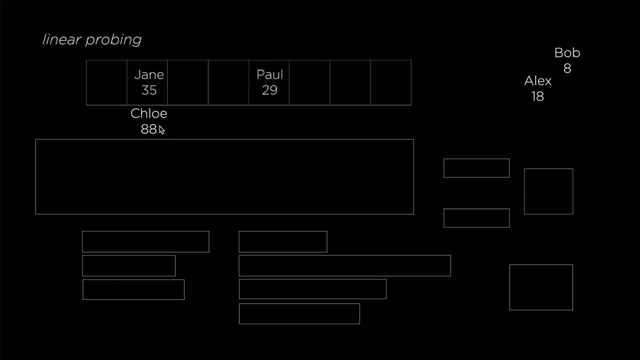 Then, with linear probing, all we need to do is we'll need to check the element that's directly to the right of the collision, And if it's empty, we can just put it there. And if another element collides with this, one again. 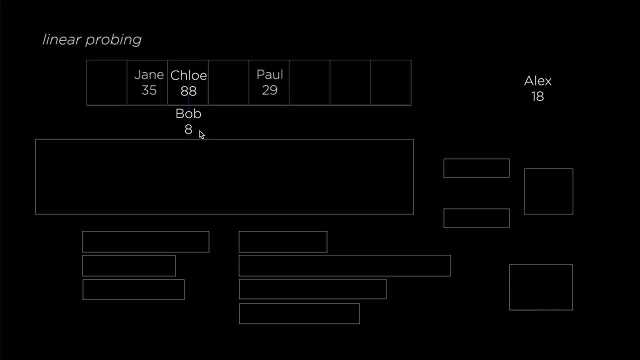 we'll need to check this element and then this element next, until we find an empty element, And then we can put it in there. So, just like that, if this new key value pair collides with this one, we'll need to keep checking the elements to the right. 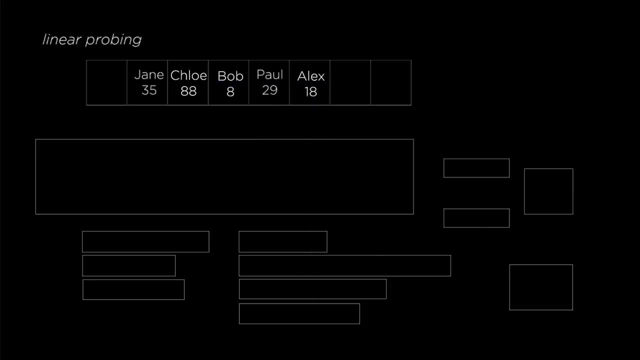 until we find an empty one. So I would say linear probing is an okay approach, but it could be inefficient when you have a lot of elements, And that's because these elements are likely to start forming clusters when you have a lot of them. 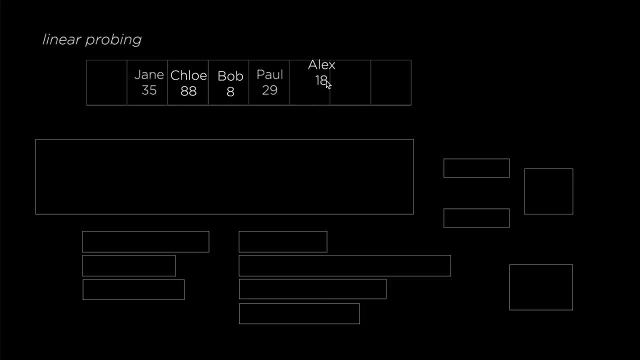 So, for example, you have a cluster of five elements here, and when you have a cluster of five elements, or maybe a lot more elements, it would take extra time to go through all of them and to find an empty spot, And one way to solve that issue is called double hashing. 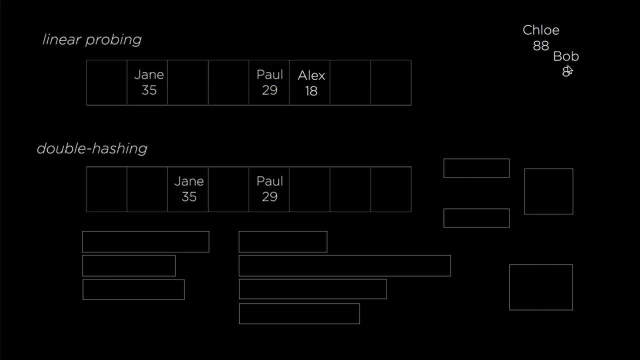 So let me explain how double hashing works. Let's say that this key value pair happens to collide with this one. Then what we are going to do is similar to linear probing, in a way that we're going to jump ahead and check other elements to see if they're empty. 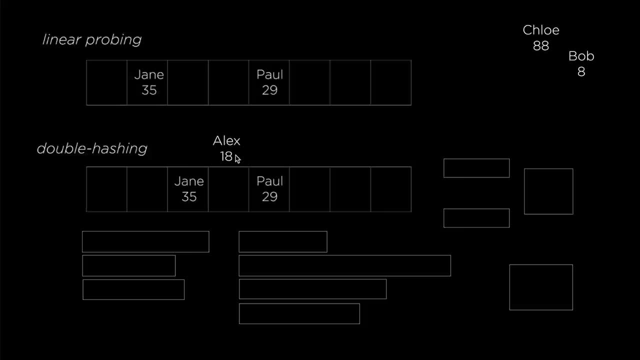 But instead of jumping ahead by one element, we're going to pick a number here, let's say three, to determine how many elements we want to check ahead. So if we pick three here, we're going to check one, two, three. 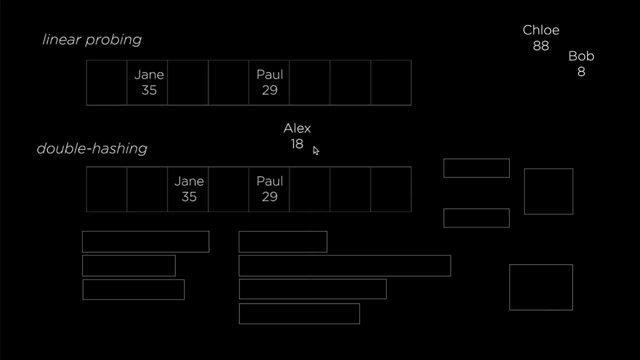 this element, the third element, and we're going to check every third element ahead of that. So, since this is empty, we're going to put it here, But if another pair collides with this one and if we happen to pick three again, 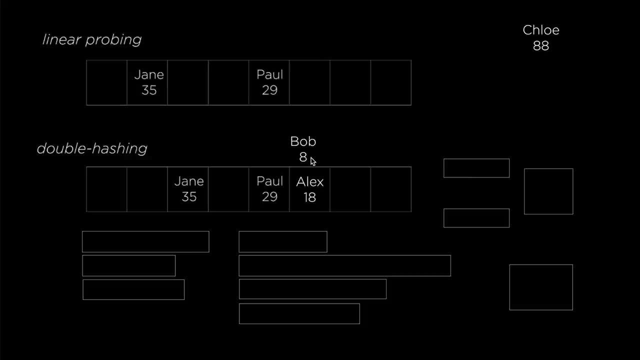 we're going to check the third element and then we're going to jump ahead by three elements again. So that would be one, two, it would be this element, but since it doesn't exist, we're going to jump back here. 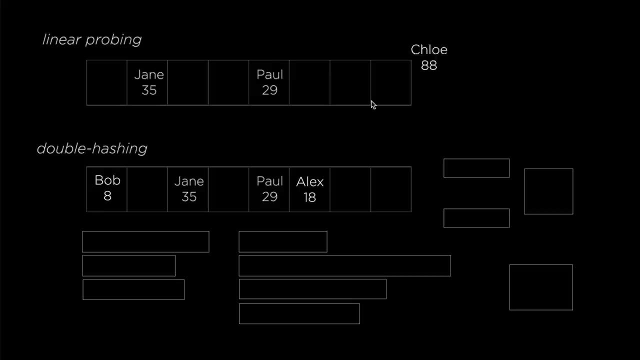 And the nice thing about double hashing is that every time we have a collision, depending on the key or depending on the starting point, we're going to produce a slightly different sequence every time, the sequence of the elements that we're going to check. 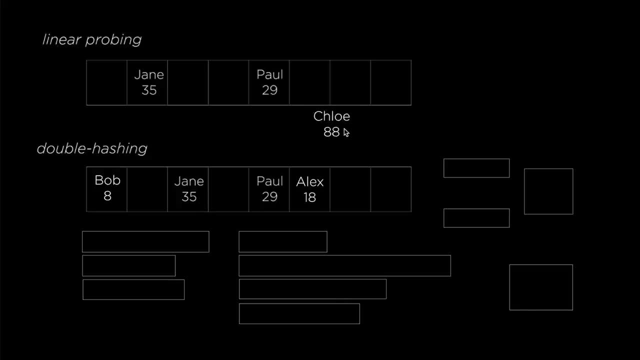 So let's say that this new pair collides with this one. we might pick one for the number of elements that we're going to jump ahead. If we pick one, we're going to just go to this element and find that this is empty. 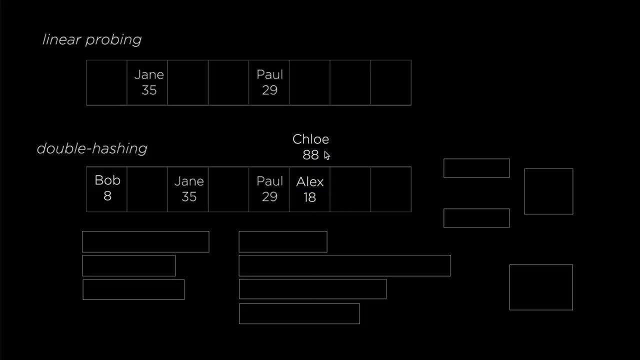 So we don't necessarily jump from here to here and have another collision, And that's why we're less likely to have clusters in double hashing and that's why it can be more efficient than linear probing. To summarize this: we first pick our initial index. 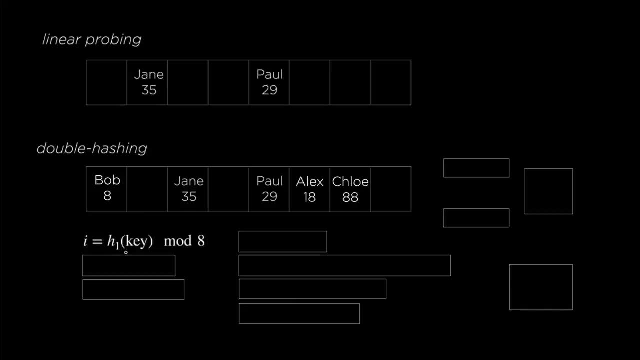 for the given key with a hash function- h1, with the model operator the length of the array, in this particular case, 8.. And then the next index that we're going to check is going to be the original index plus c, the number that we're going to pick. 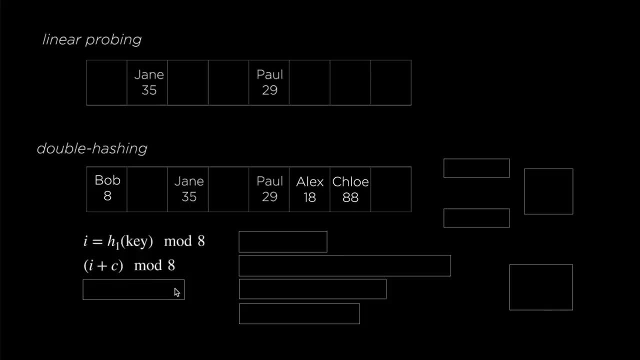 for the particular key, mod 8.. And the next one after that is going to be i plus 2c, mod 8, and so on. And here I think the natural question would be: how do we pick this number c? 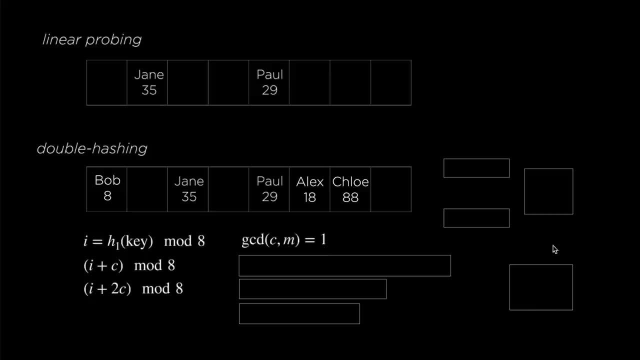 Well, one condition that we need to satisfy is that gcd of c and m, or the greatest common divisor, or the greatest common factor of c and m, should be 1.. And m is the length of the array here. And that's because, by satisfying this condition, 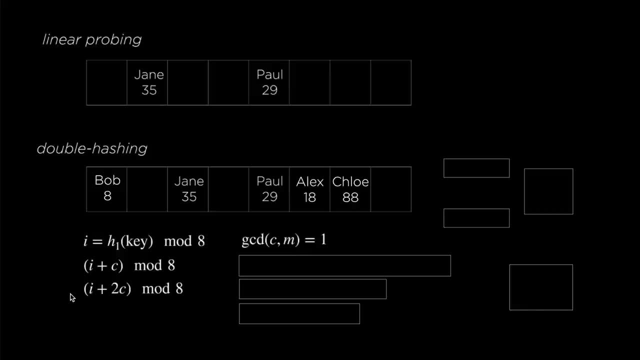 we can make sure that this sequence of indices will eventually cover the entire array, And one convenient way to make sure that's true is to always set m- the length of the array- to be a prime number and c to be a positive integer. 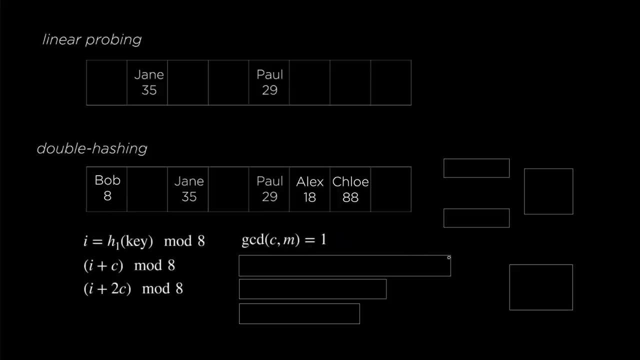 And that way, gcd of c and m will automatically be 1.. Okay, so how do we pick c? Here's one way of picking it. assuming that m is a prime number, We're going to use a second hash function, which we're going to call h2,. 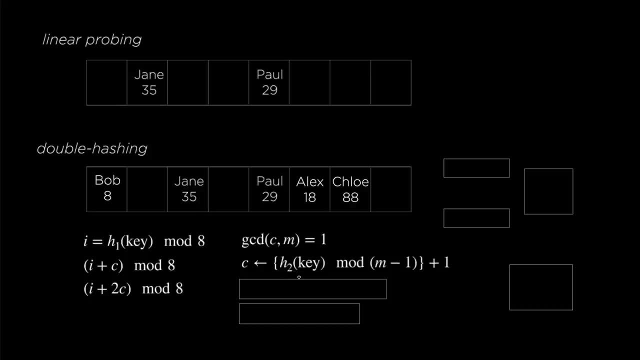 and then we're going to put a key into that function and then do some operations here. So let me explain what we're doing here. Here we're applying the mod operation with m-1 to the result of the hash function, And that way. 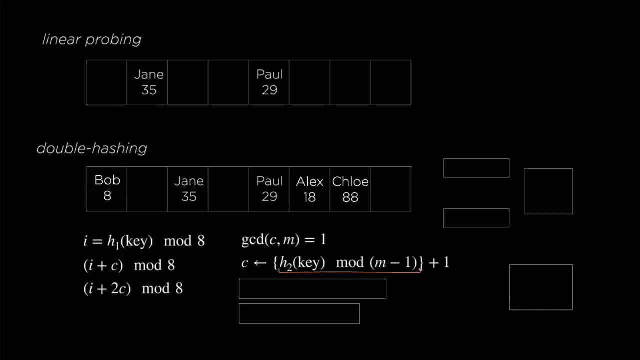 the range of the results that we can get from this whole expression is going to be 0 to m-2 inclusive, And by adding 1 to that result, we're going to get the range 1 to m-1 inclusive, and that's the range that we want. 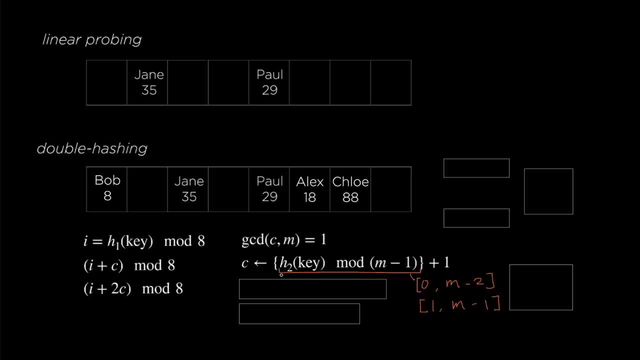 And here the natural question after that is: how do we pick h2?? For that I ran an experiment and I tried a few different approaches. So here's the first approach I tried. We have h1, the original hash function, and to make h2, 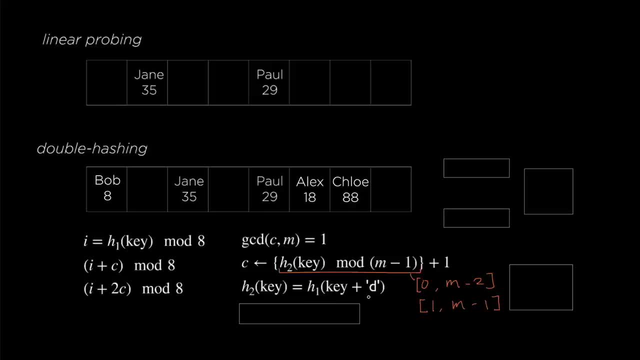 I simply appended a letter which I picked. it could be anything, but I picked d here to the key. So if the key is jane, I just put jane d to h1, and then I used that as h2.. And it actually seemed to perform pretty well. 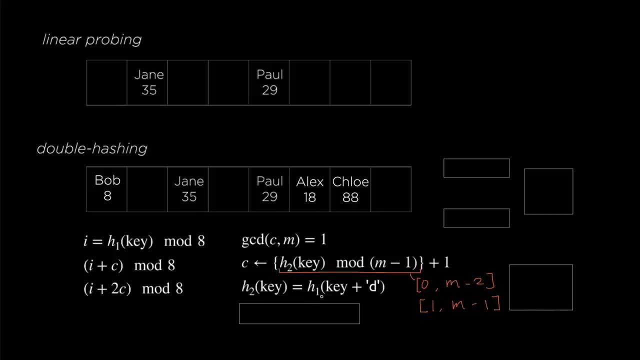 And, by the way, the h1 I used for this one is the default hash function of Python, Which seems to be based on djb2, which I mentioned earlier, And the second approach I tried is simply this, So I used exactly the same hash function. 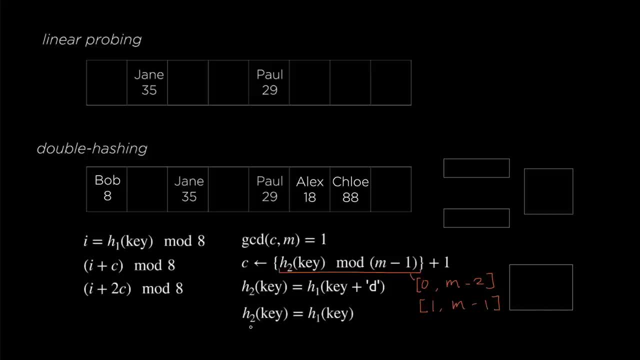 as the original one, as the second hash function And so much surprisingly, it performed as well as the first approach. But I would say, if you want to try implementing double hashing yourself, you should try a few different hash functions because the performance probably depends on your particular environment. 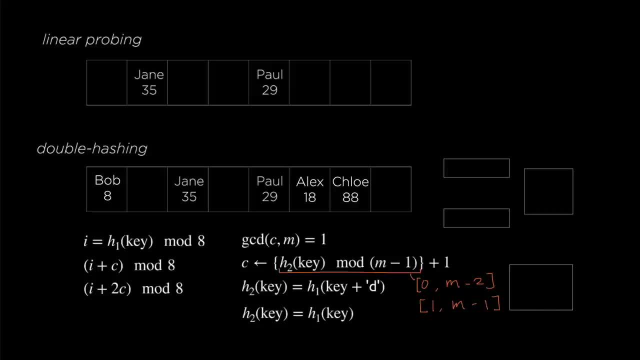 and the particular kind of input data that you get. Anyway, with double hashing you can show that, with a few assumptions, that to complete either the search operation or the insertion operation you need to check at most this number of elements. on average That's 1 over 1 minus alpha. 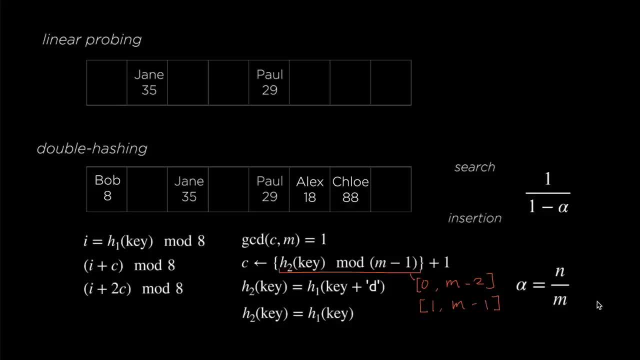 where alpha is n over m. So again, n is the number of elements that we've put in so far in the hash table and m is the length of the array. So, just like I said before, alpha shows how full your hash table is. 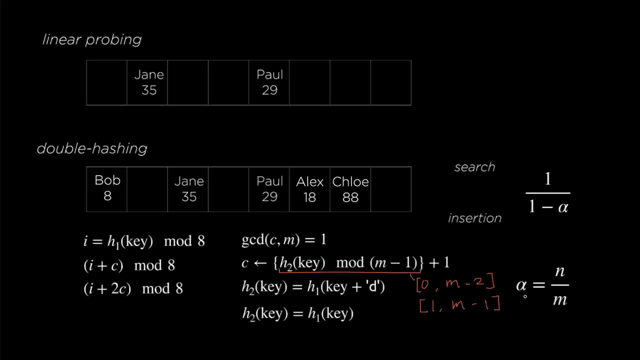 So let's say that alpha is 2 thirds. Then this expression, 1 over 1 minus alpha, becomes 3.. So that means that to complete search or insertion you need to check at most 3 elements on average. So basically, 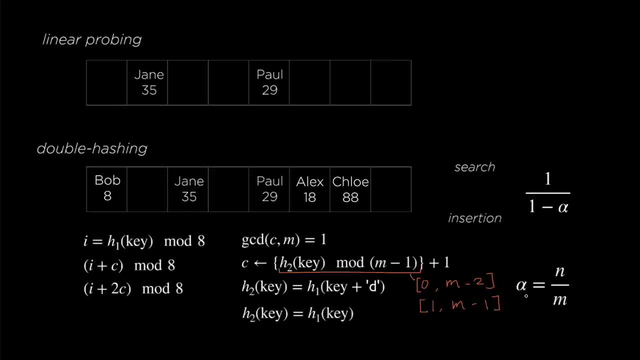 if you keep alpha below a certain number, let's say 2 thirds again, you'll be able to complete search or insertion in constant time. So what I would suggest? if you're implementing double hashing by yourself, well, at least one way to do that. 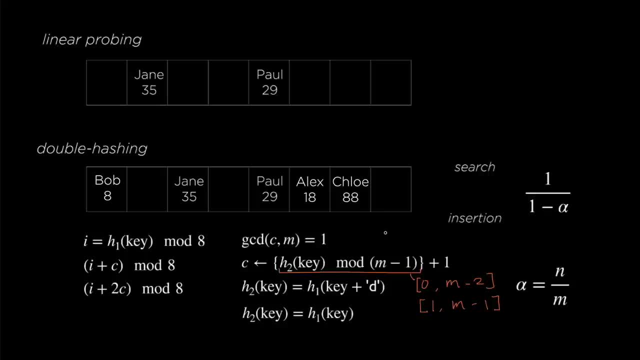 would be to pick m to be a prime number- let's say 7 or 701, and then, as soon as alpha becomes greater than 2 thirds, resize the array, pick a larger prime number than the original m and then transfer all the elements. 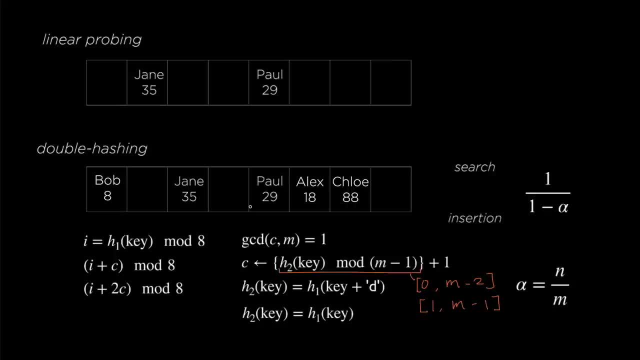 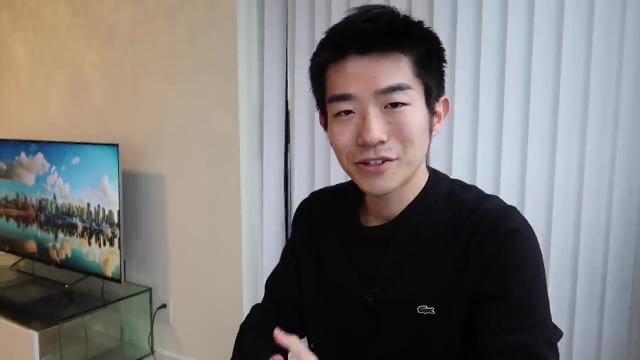 to the new array, And that way resizing the array takes extra time, but at least for search and insertion it's only going to take a constant amount of time as long as alpha stays low enough. OK, so that's my introduction. 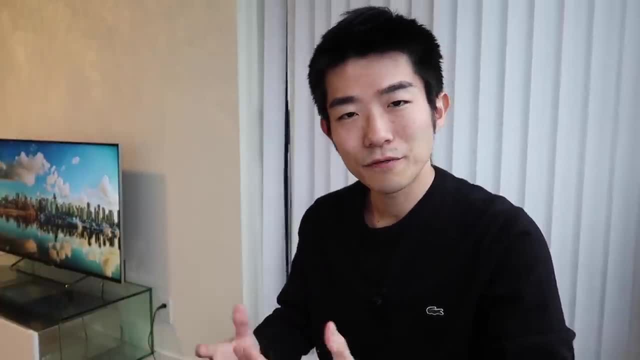 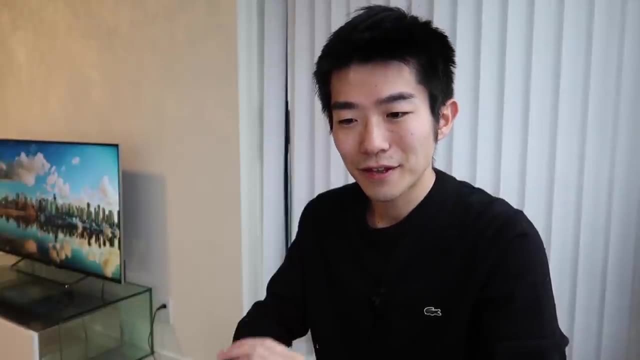 to hash tables and dictionaries. but there are a few things I wanted to mention before I go. One is that there is a coding interview problem that I covered a while ago on this channel, and for that problem you can actually use one of these concepts. 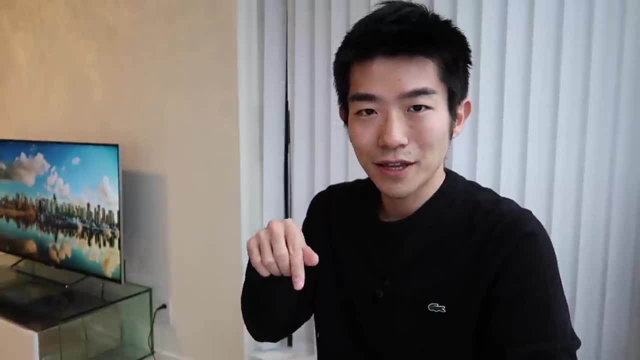 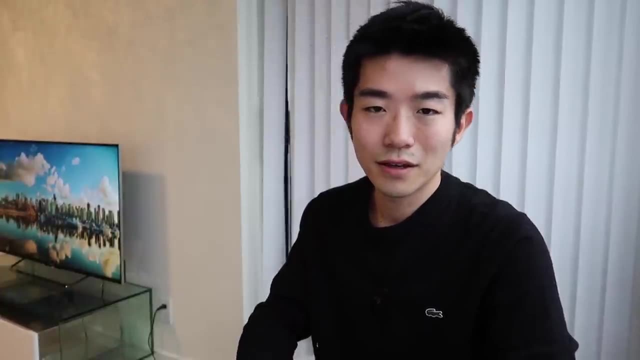 to solve it, So I'll put a link to that video in the description below, just in case you want to watch it. The other one is that I tried implementing a hash table in Python, so I'm going to put a link to that code. 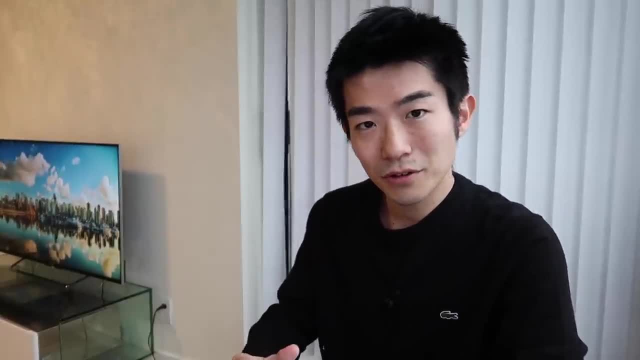 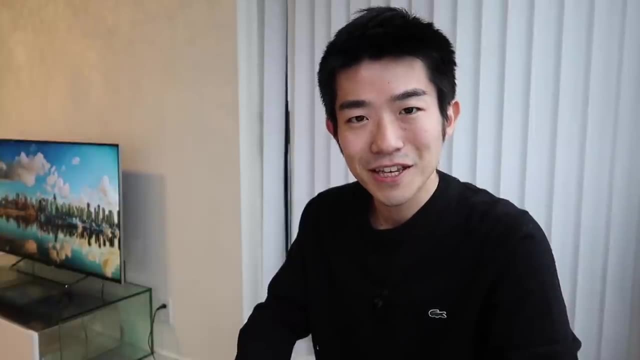 in the description below as well, And from that code you'll be able to see how I ran the experiment I mentioned earlier too. Anyway, thank you, as always, for watching my videos, and I'll see you guys in the next one.